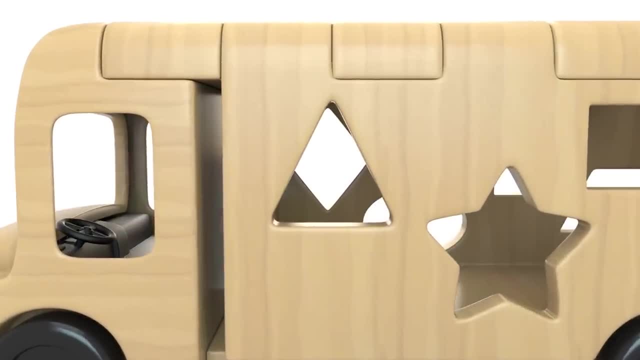 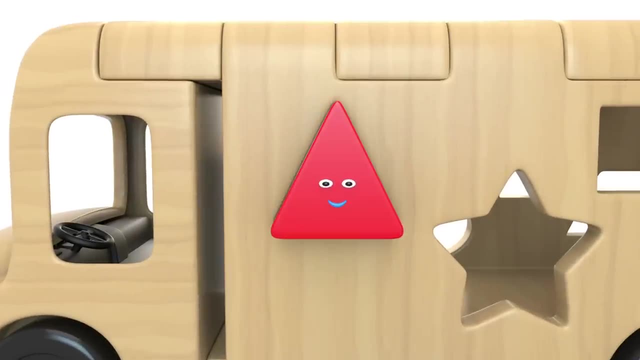 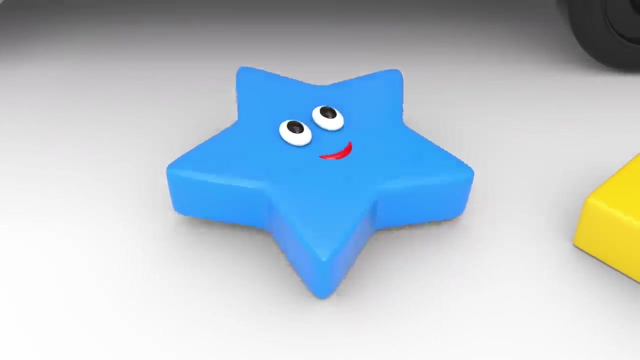 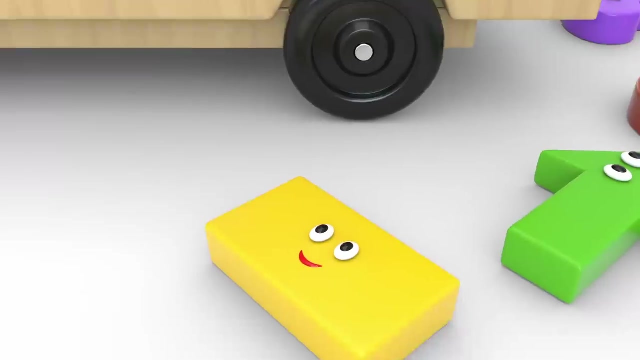 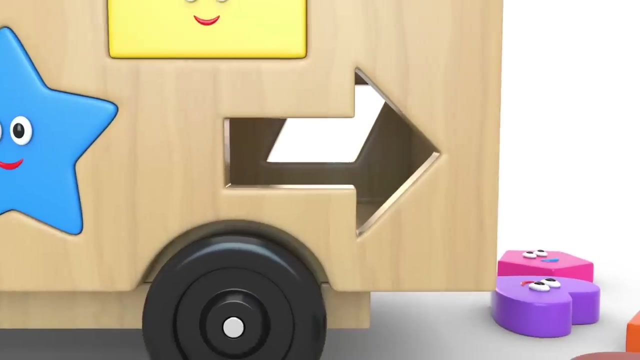 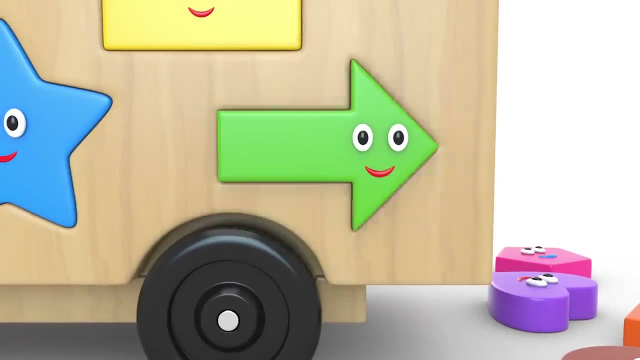 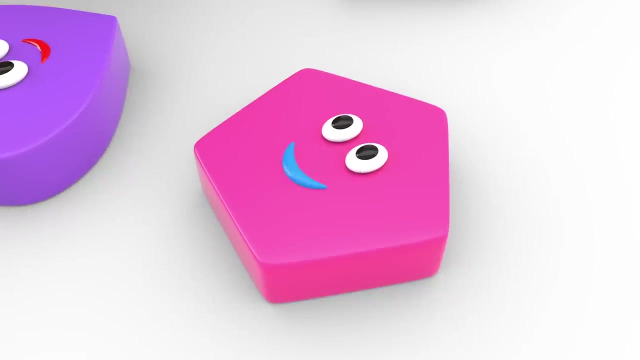 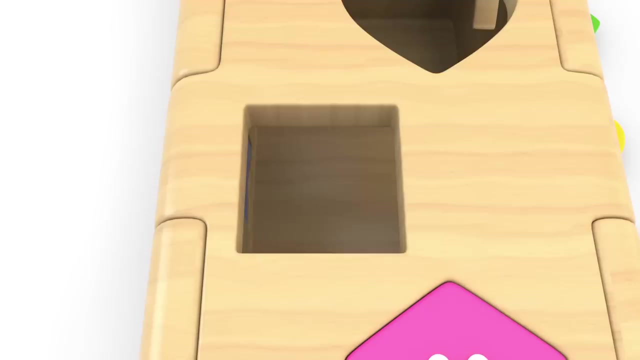 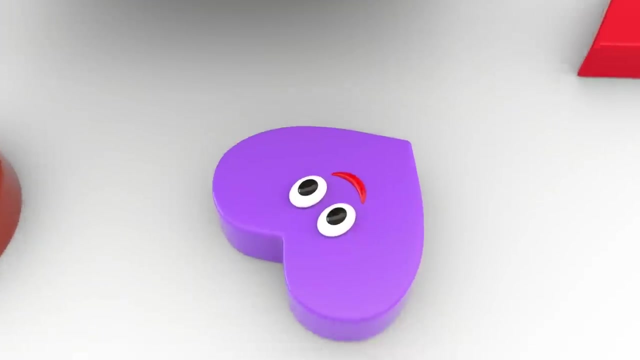 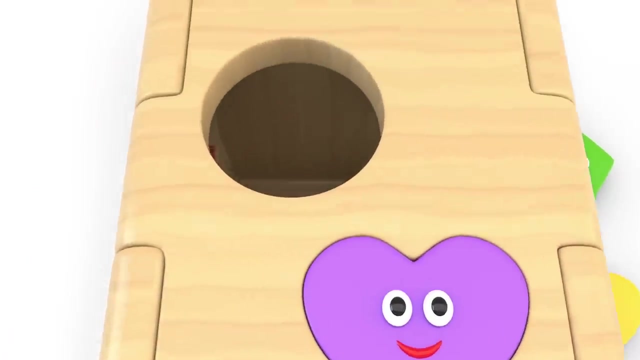 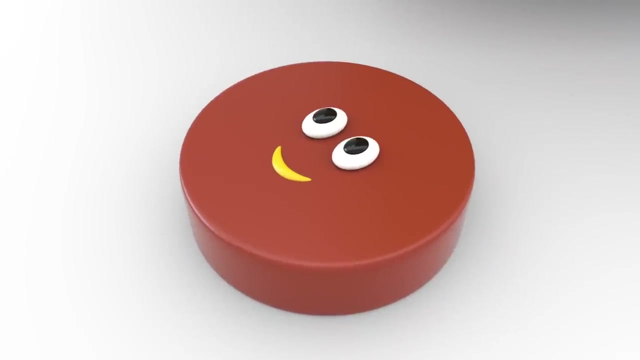 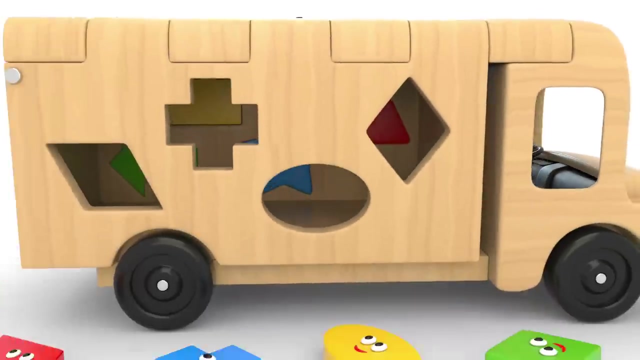 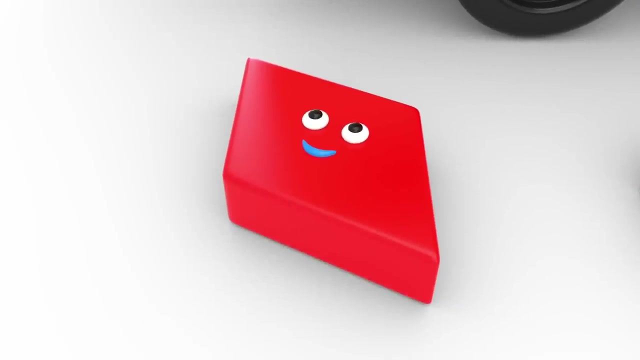 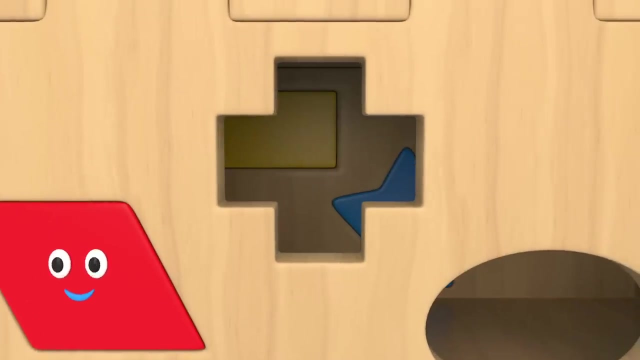 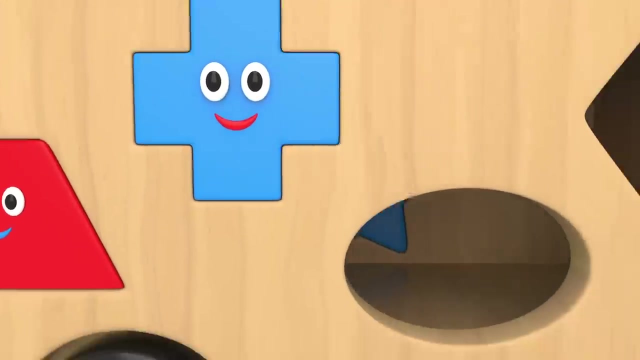 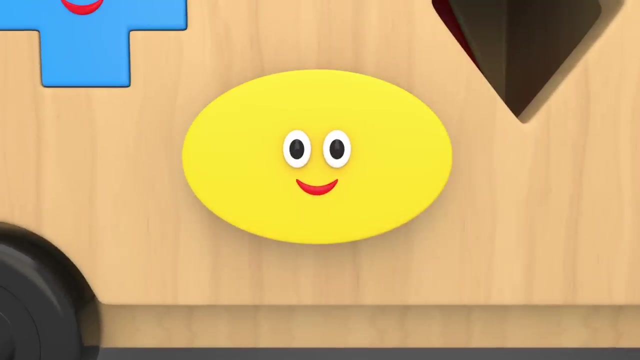 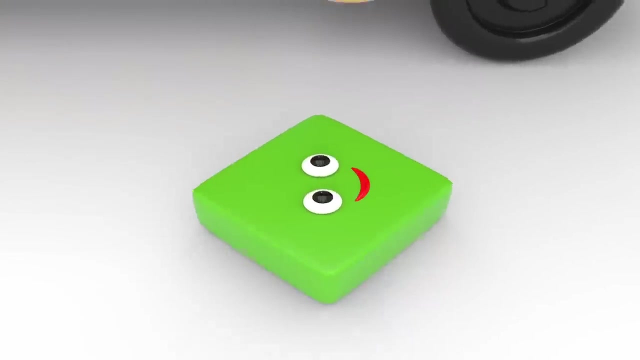 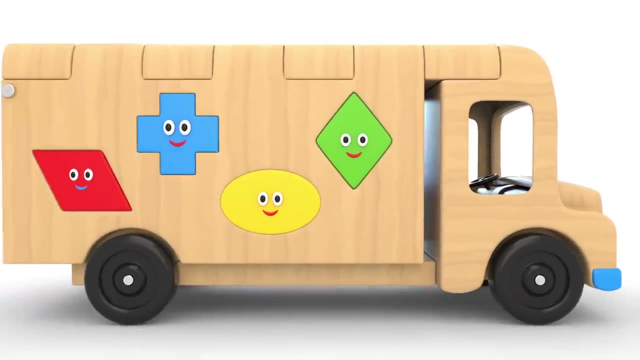 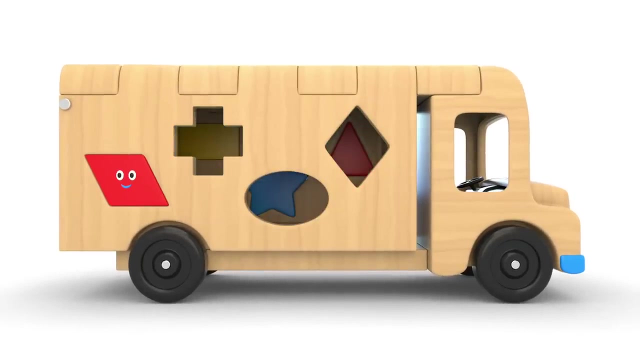 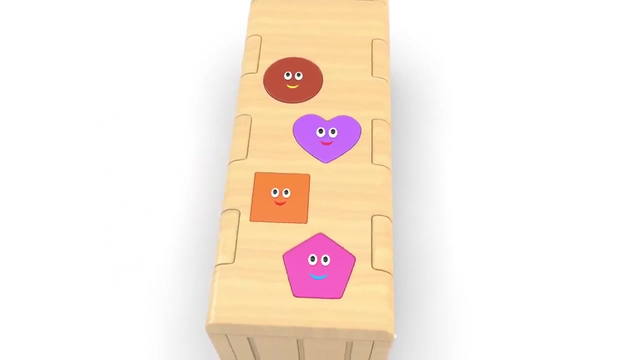 Triangle, Star, Rectangle, Arrow, Pentagon, Square, Circle, Square Heart Circle, Parallelogram, Parallelogram, Parallelogram, Cross, Cross, Cross, Oval Oval Cross, Oval Oval, Oval, Oval, Oval, Oval Oval Cross, Cross Cross, Parallelogram, Parallelogram, pentagon, square heart circle. 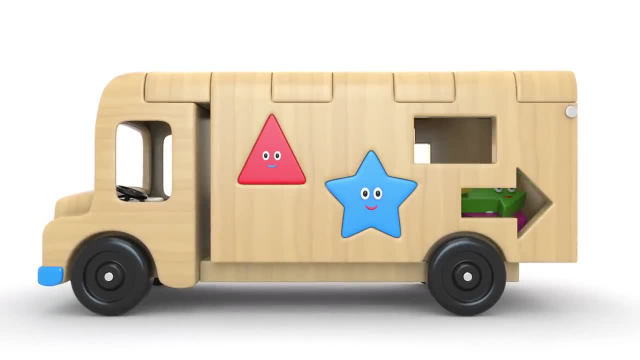 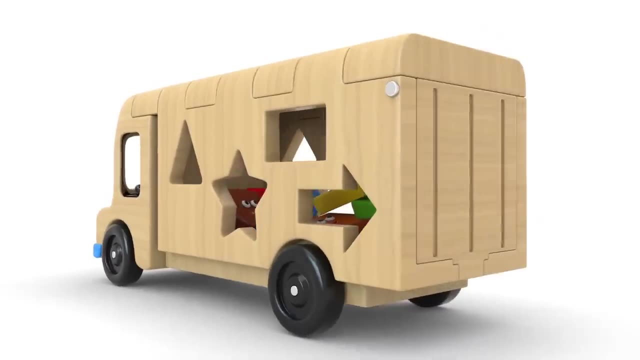 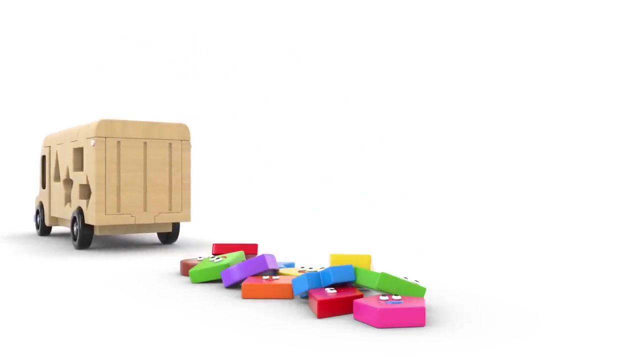 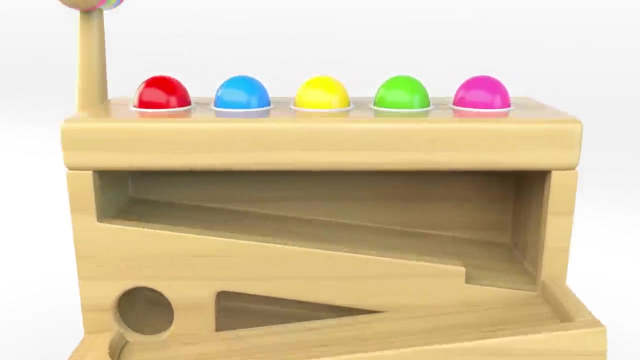 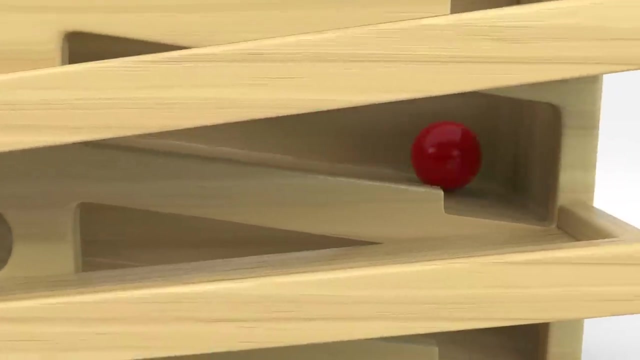 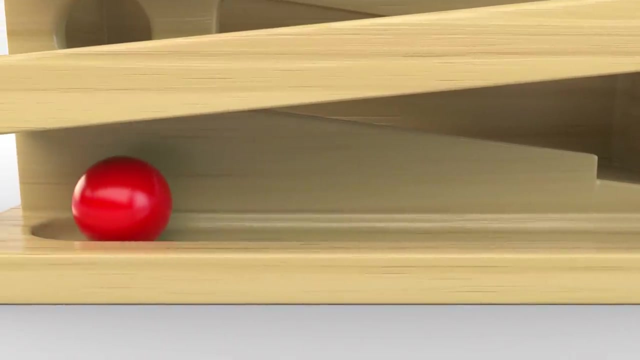 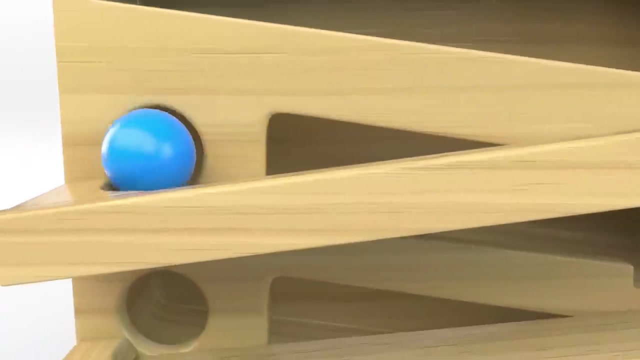 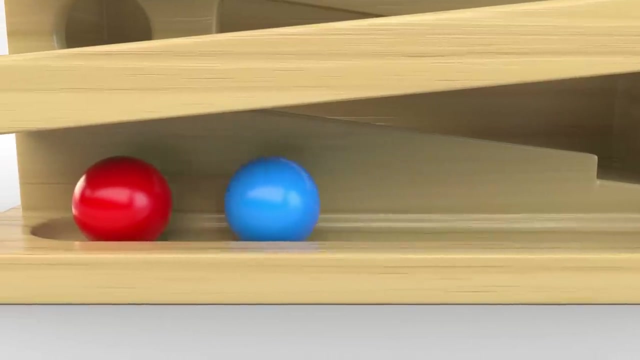 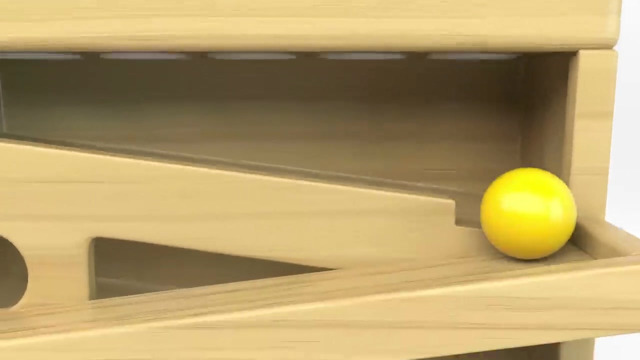 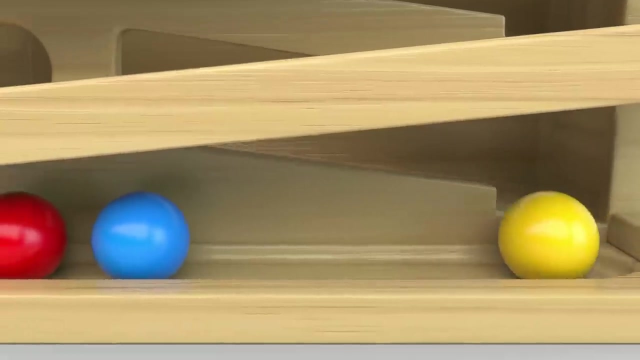 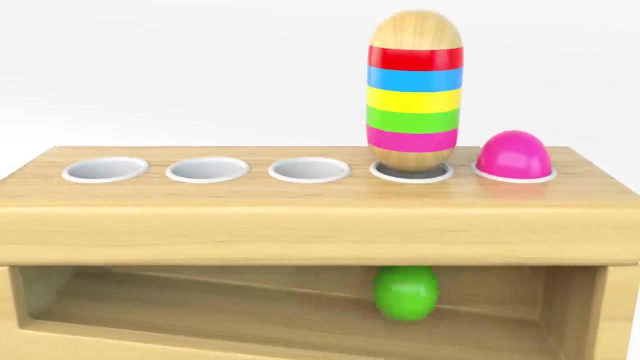 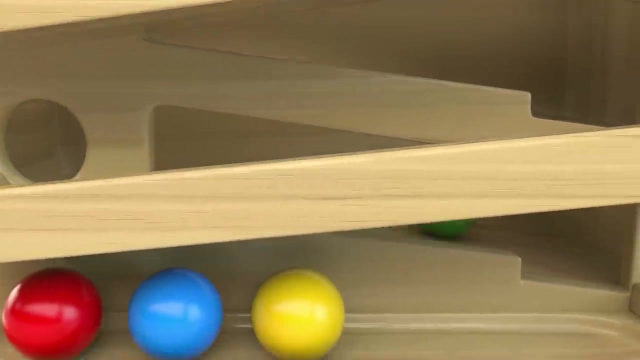 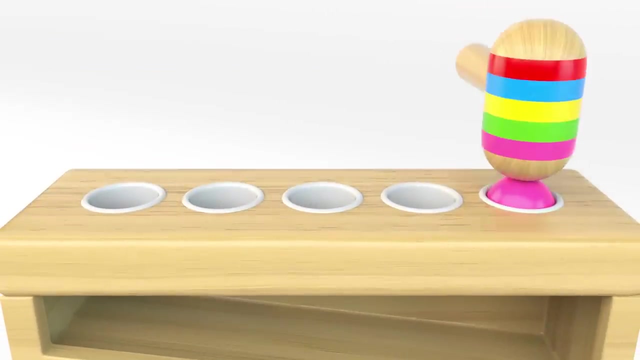 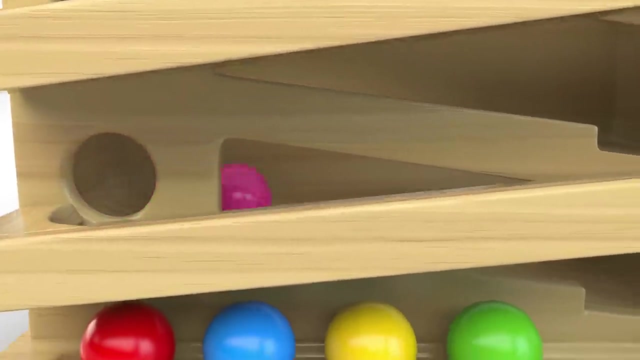 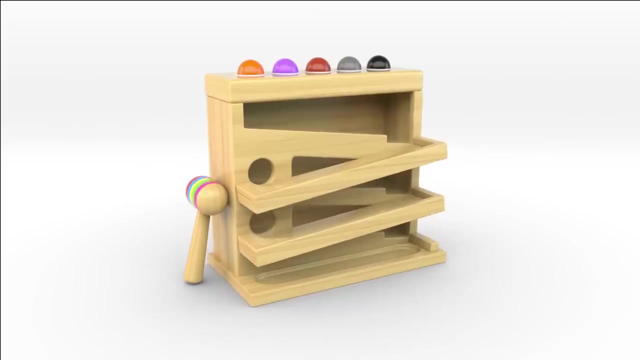 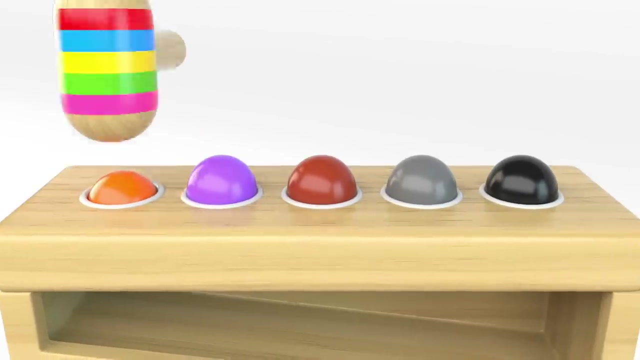 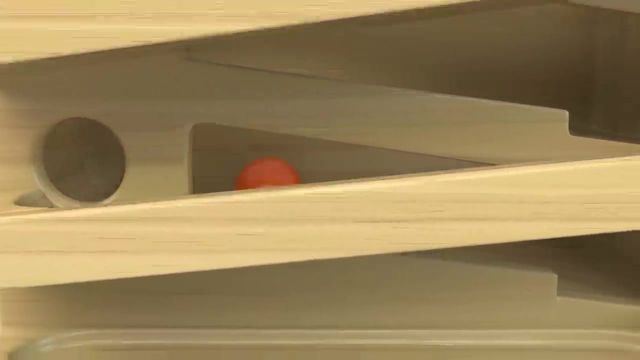 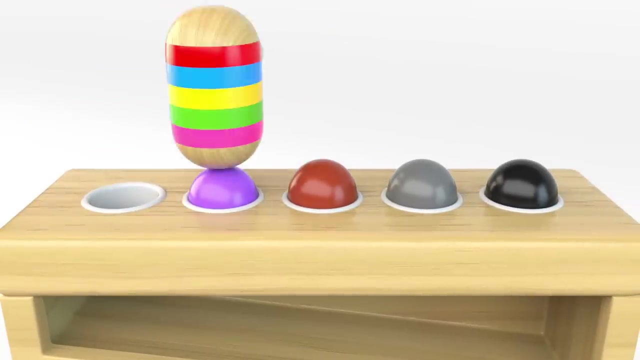 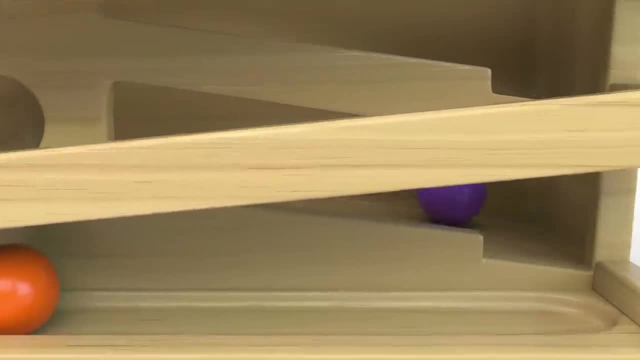 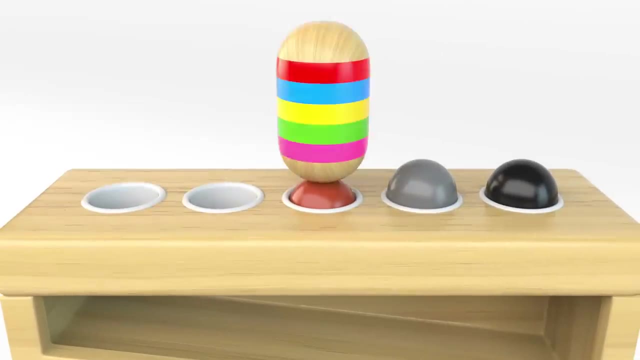 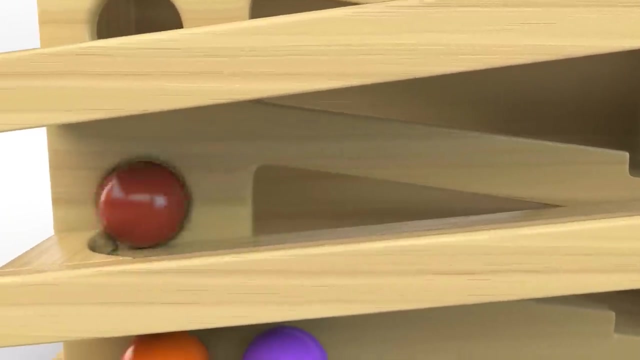 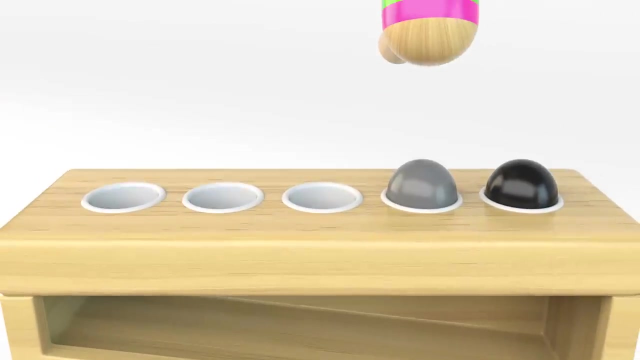 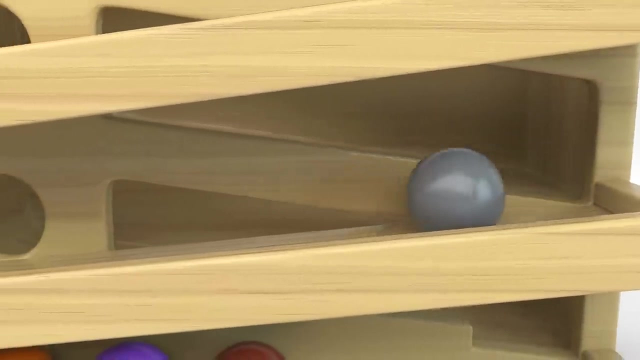 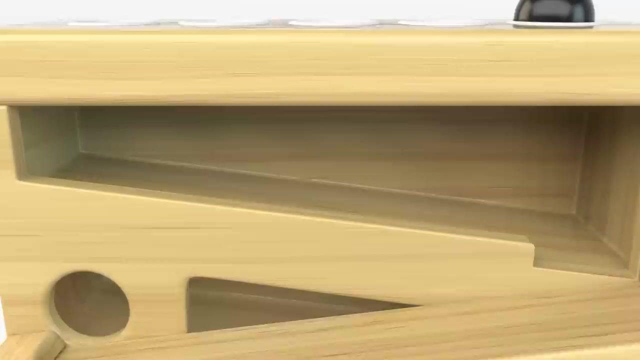 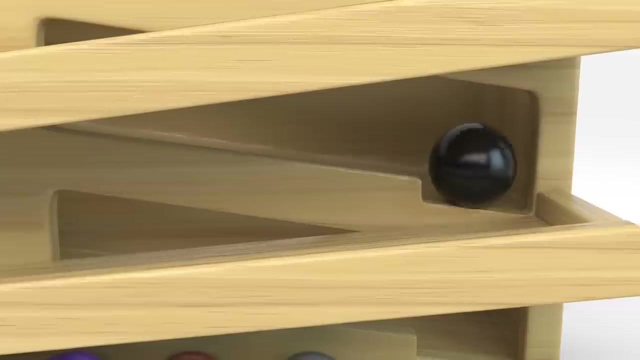 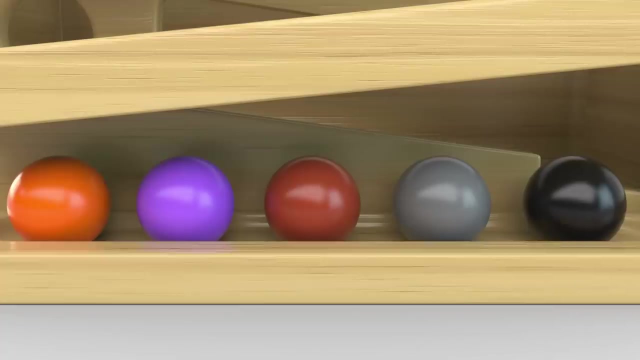 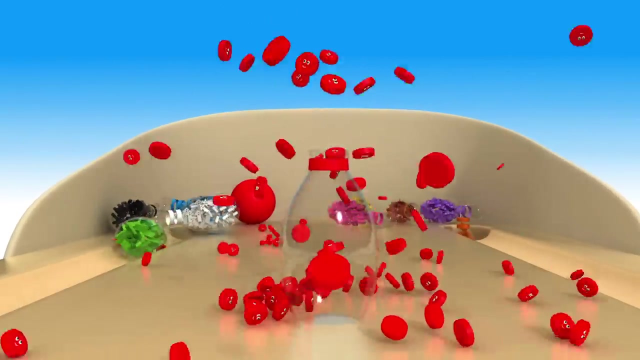 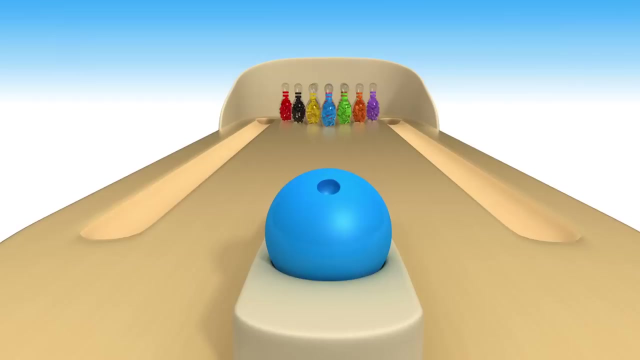 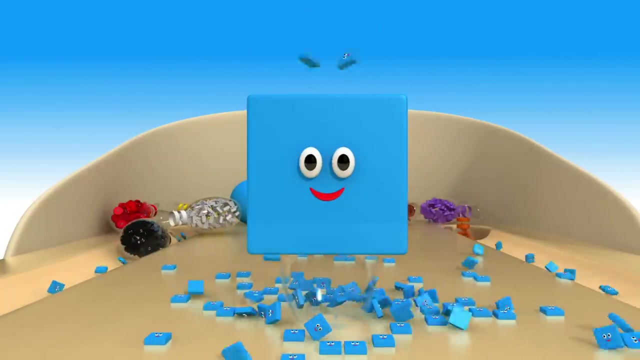 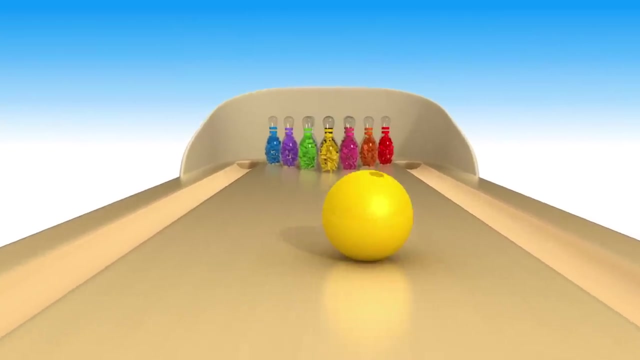 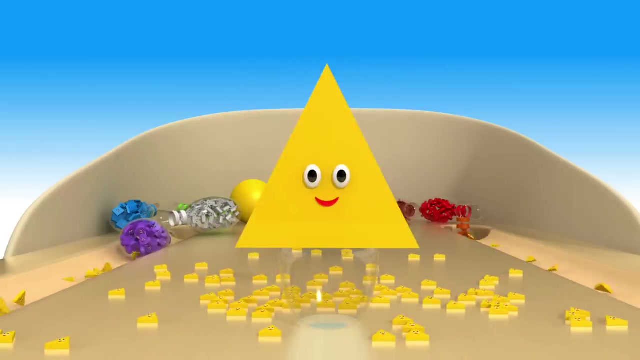 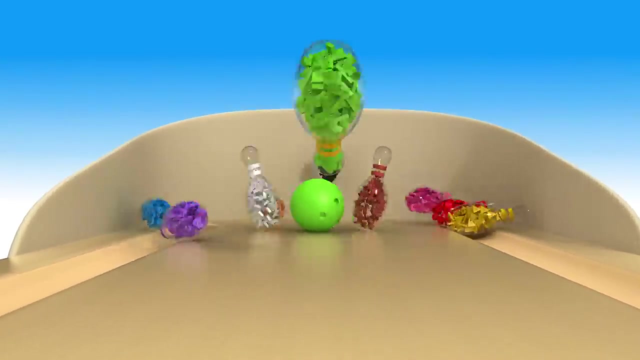 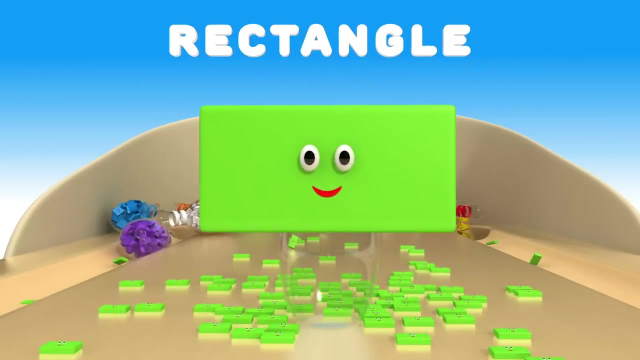 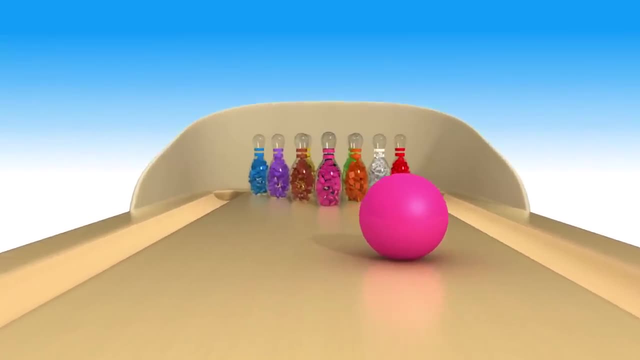 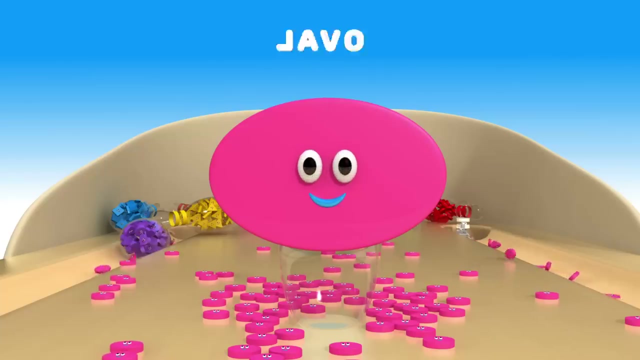 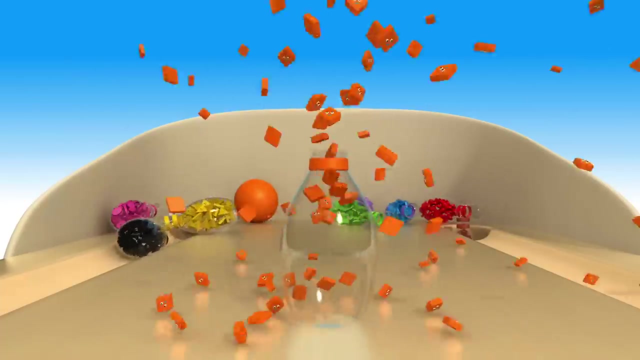 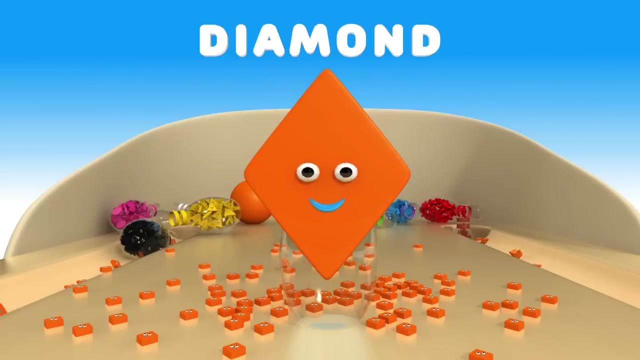 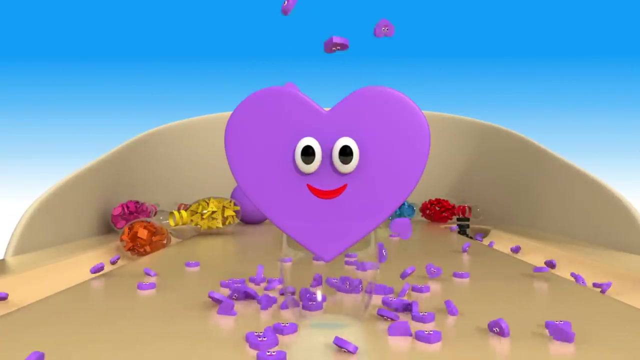 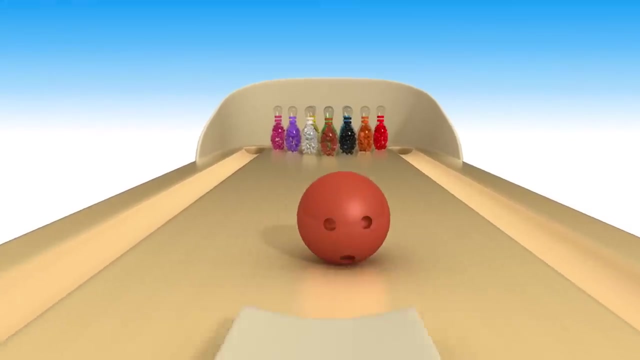 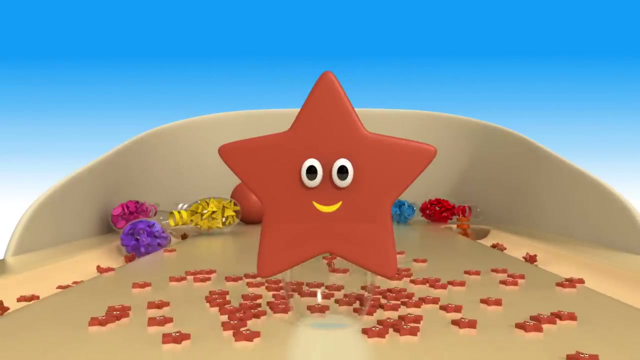 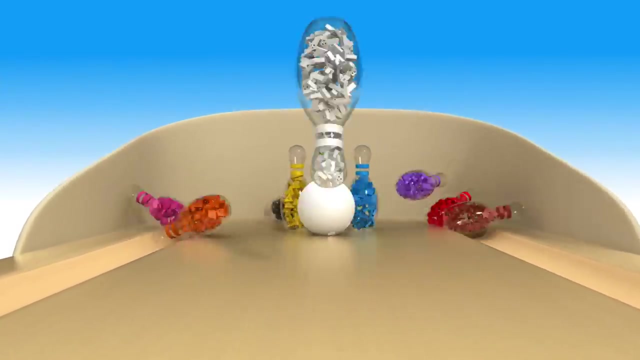 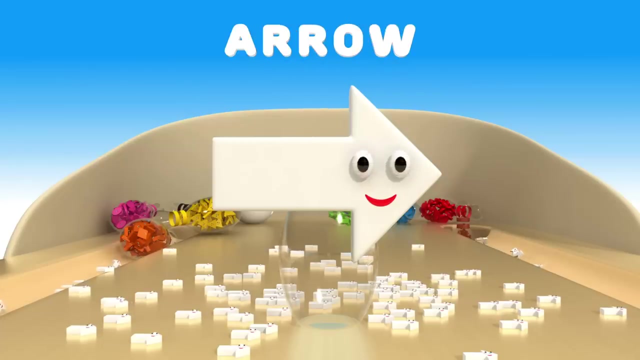 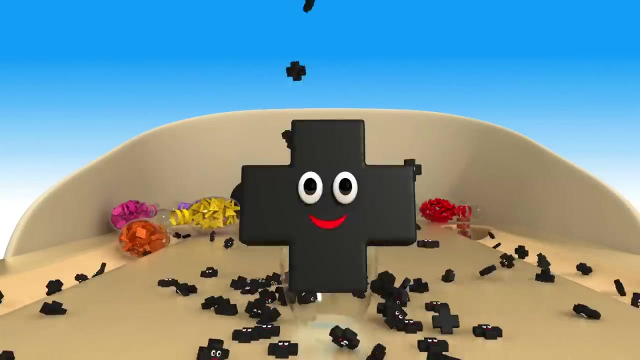 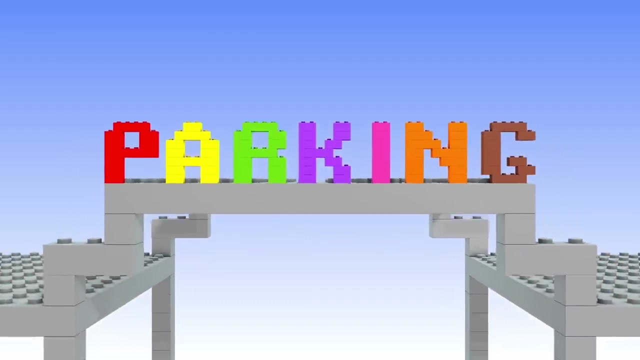 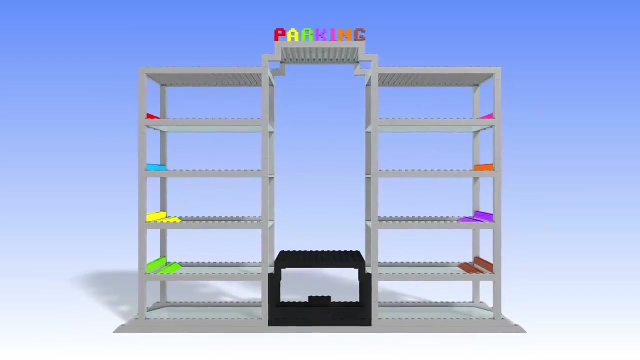 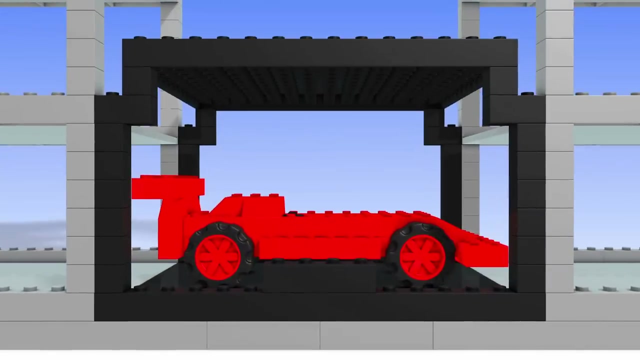 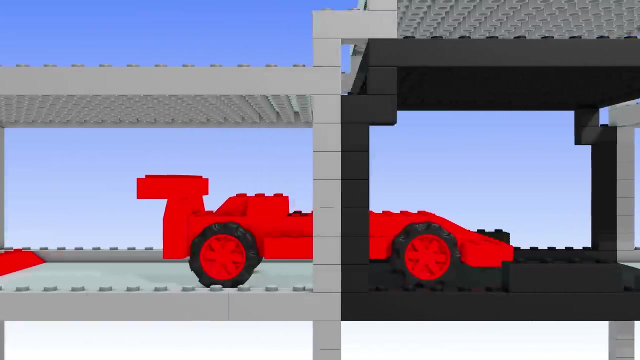 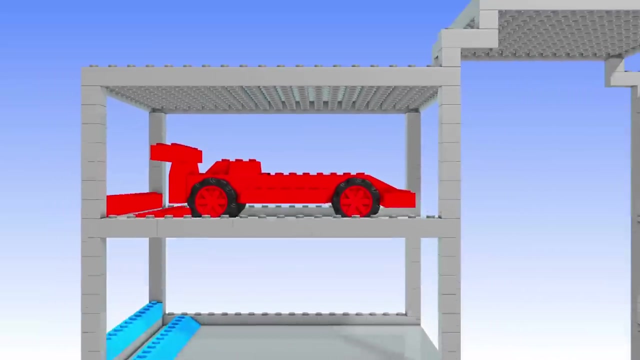 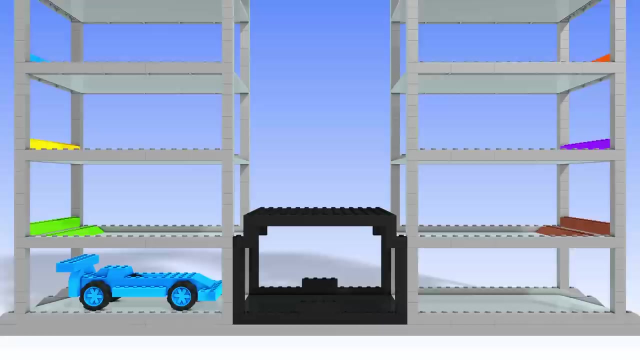 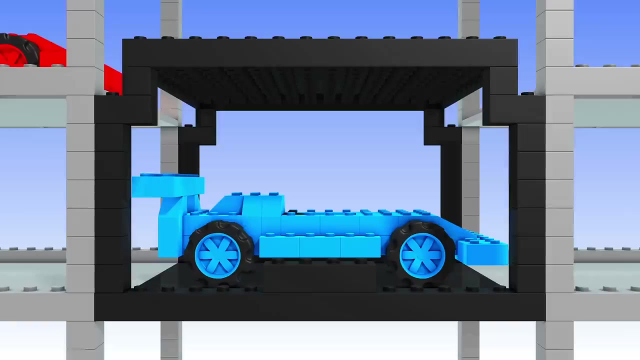 rectangle: pink, pink, wow, oval. oval, orange, orange, orange, orange, diamond, diamond, diamond, purple, purple, wow, heart, heart, heart, brown, brown, wow, star, star, star, white, white, white, blue, blue, blue, brown, brown, pink, yellow, pink, blue, pink, blue, purple, blue, purple, blue, pink, blue, blue, green, Red, Red, Blue, Blue. 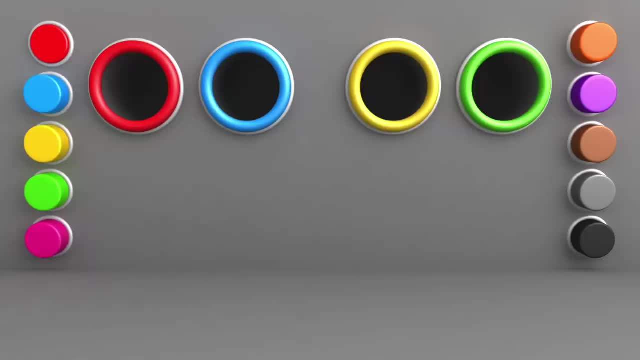 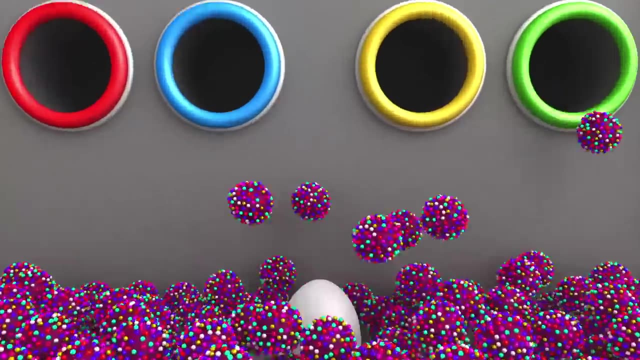 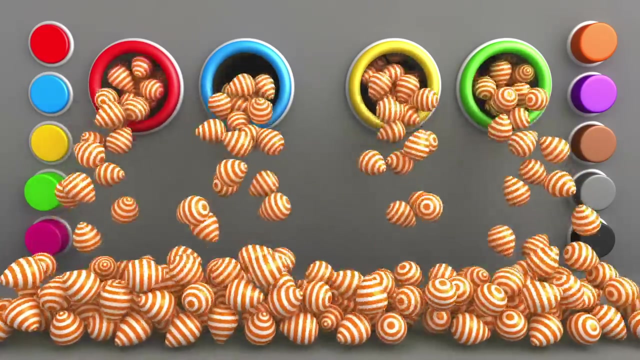 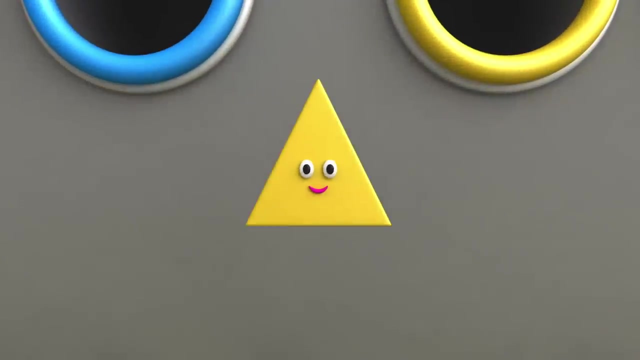 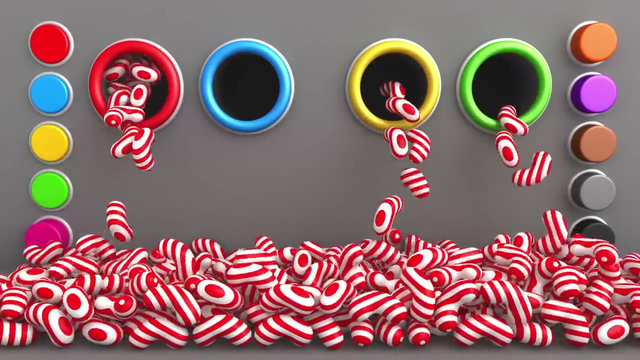 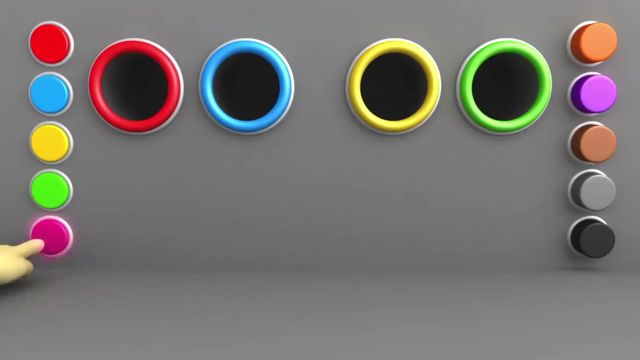 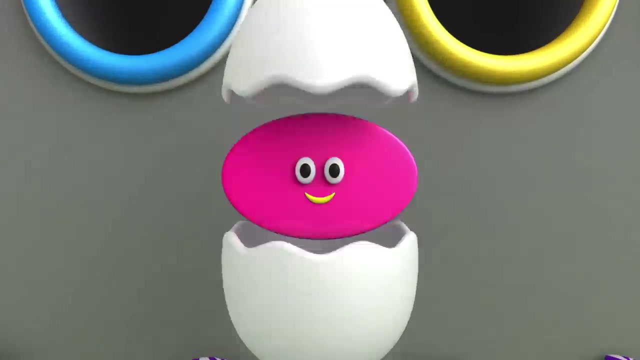 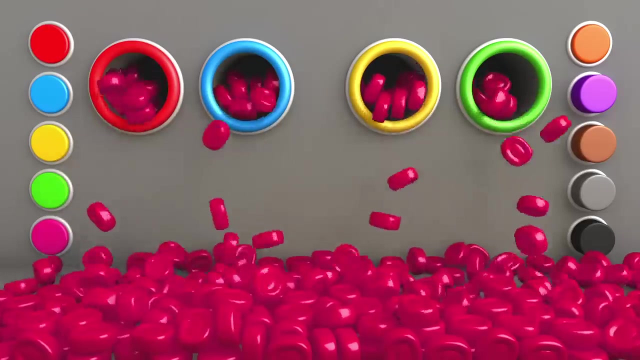 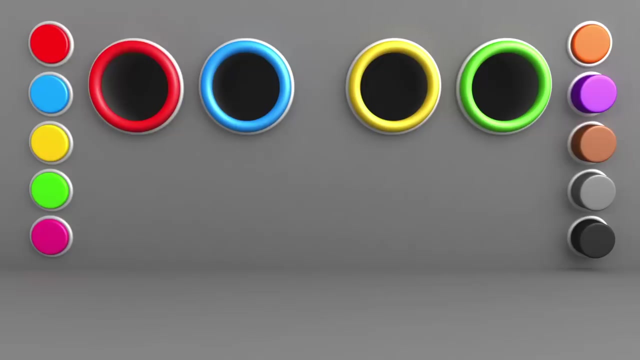 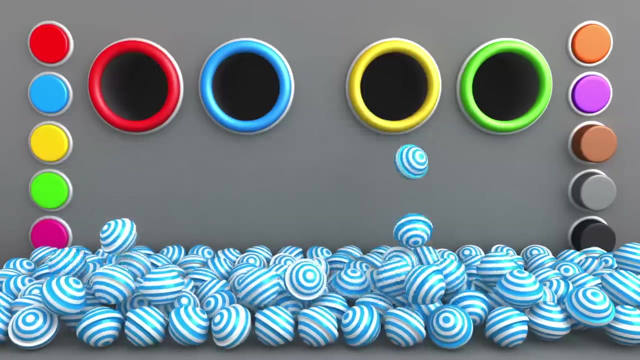 Surprise Circle, Wow Yes. Surprise Square, Wow Yes. Surprise Triangle, Wow Yes. Surprise Rectangle, Wow Yes. Surprise Oval, Wow Yes. Surprise Cross Cross, Wow Yes, Yes, Surprise Rhombus, Rhombus. 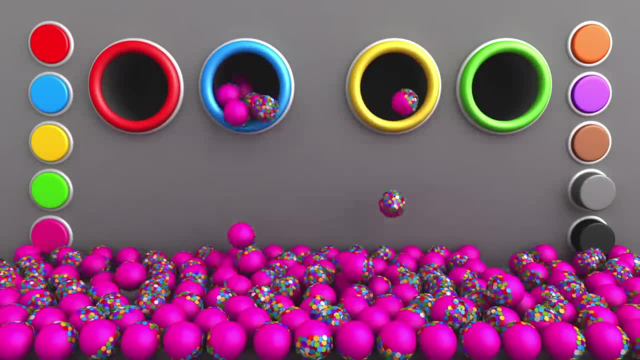 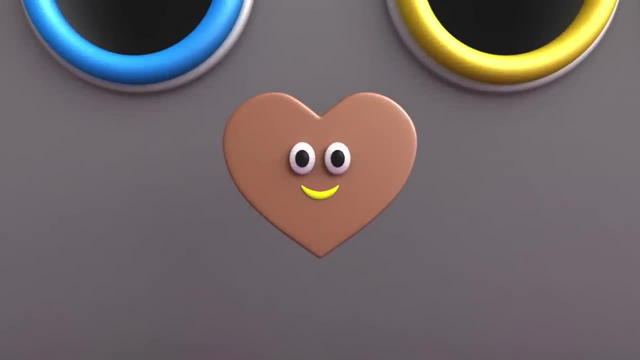 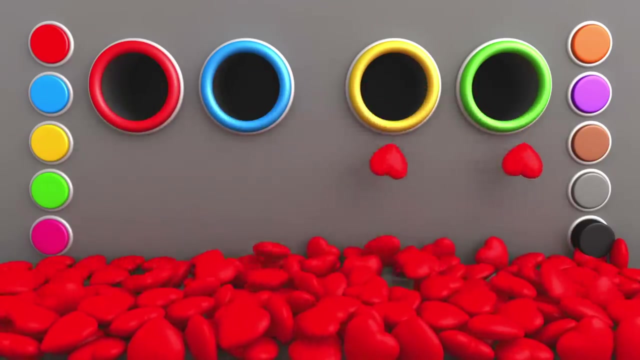 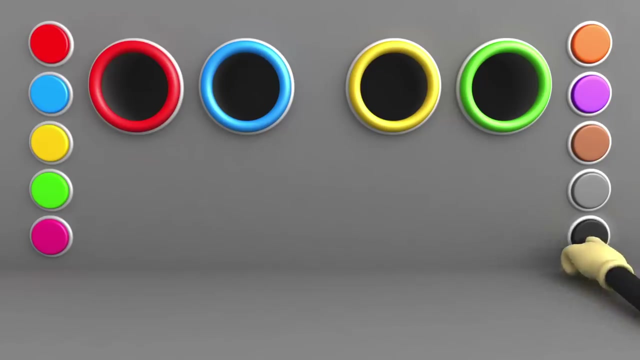 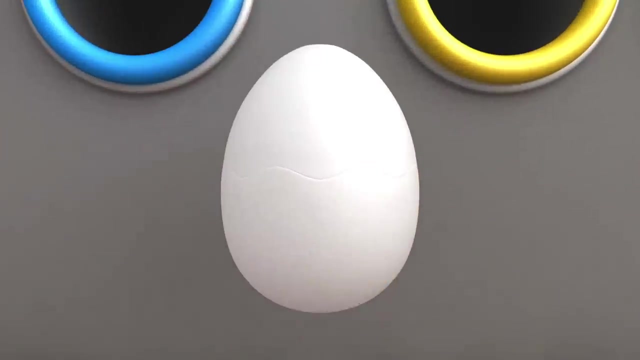 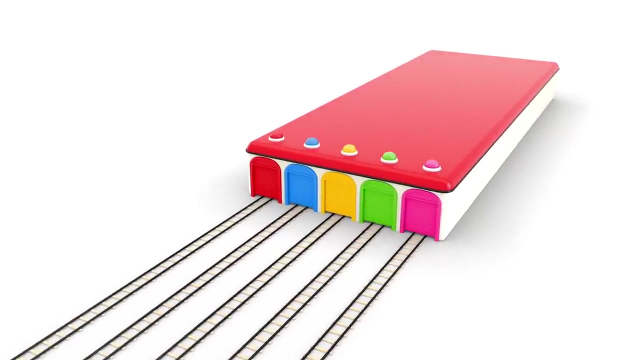 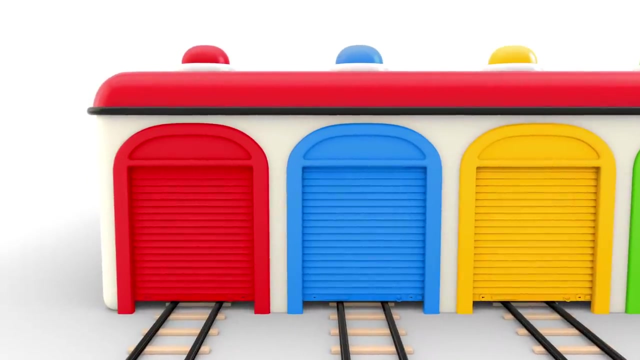 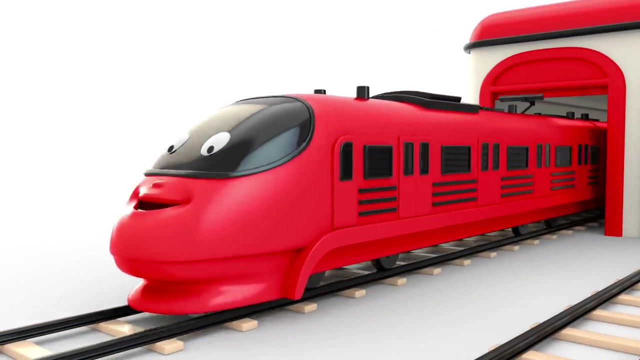 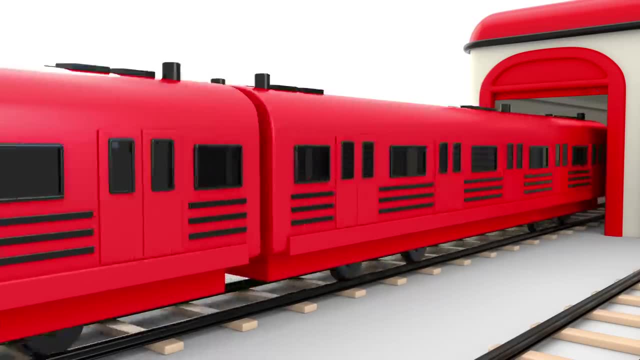 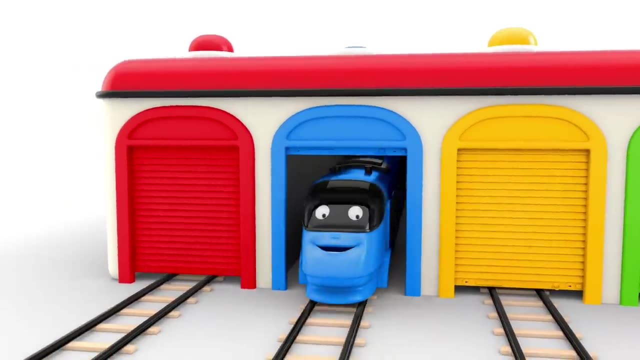 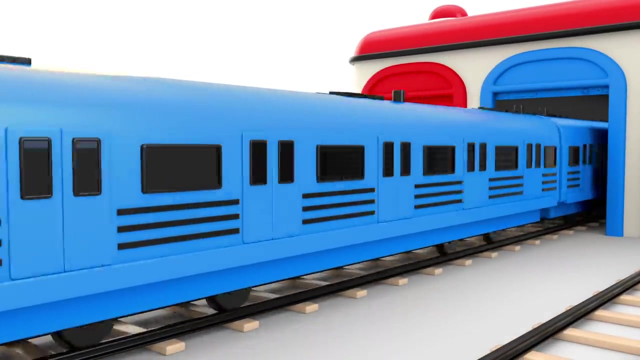 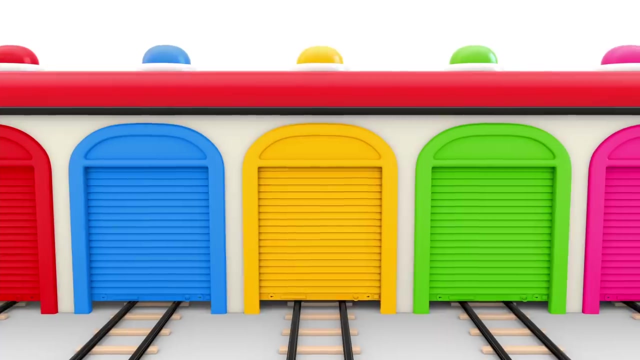 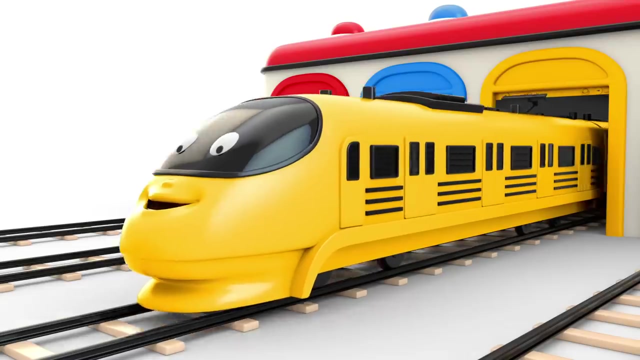 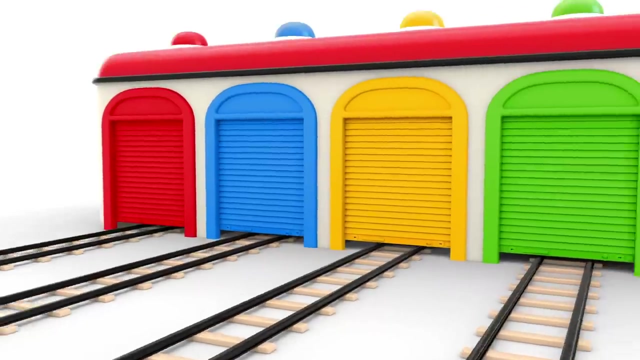 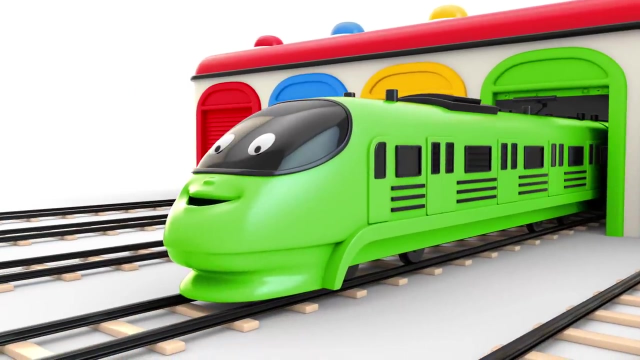 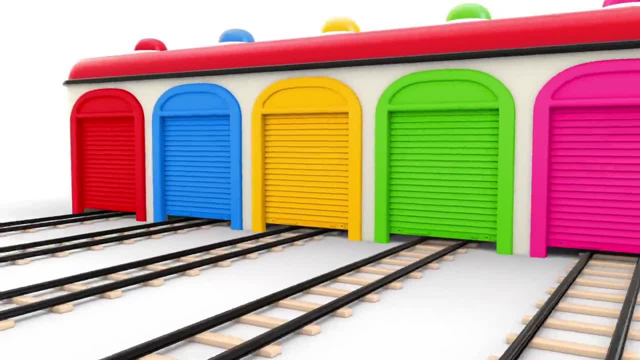 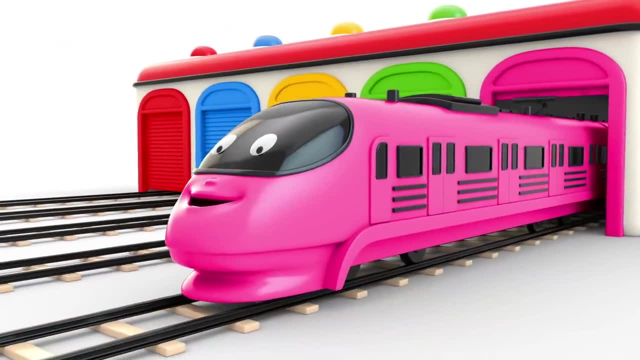 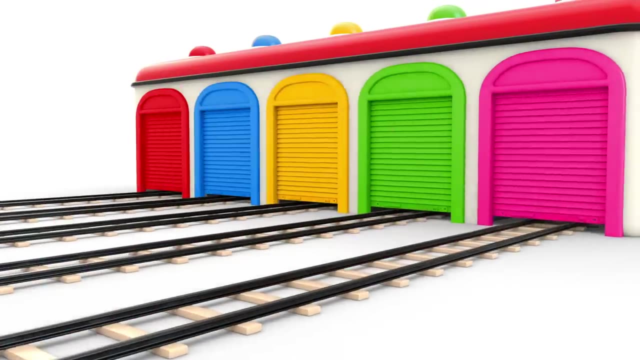 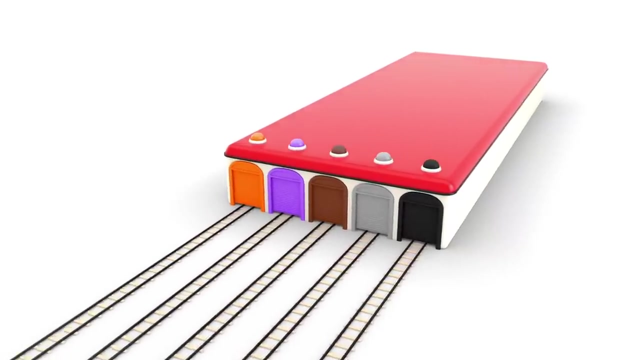 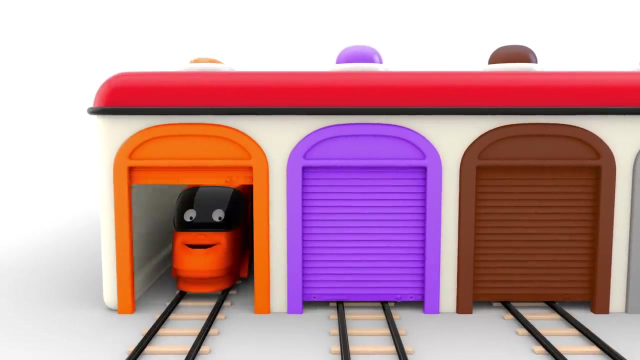 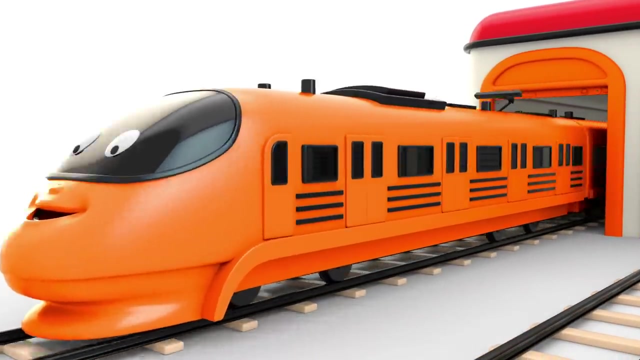 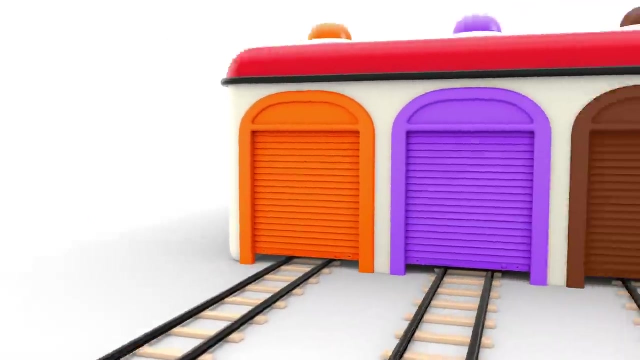 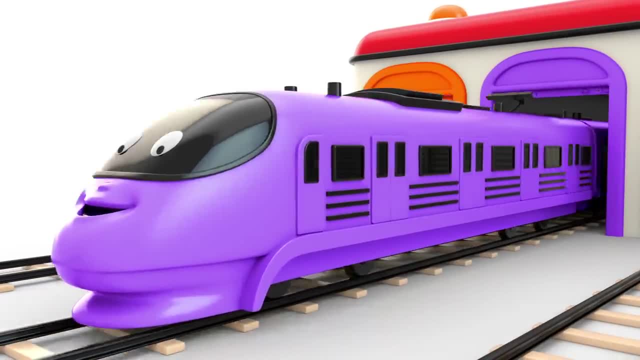 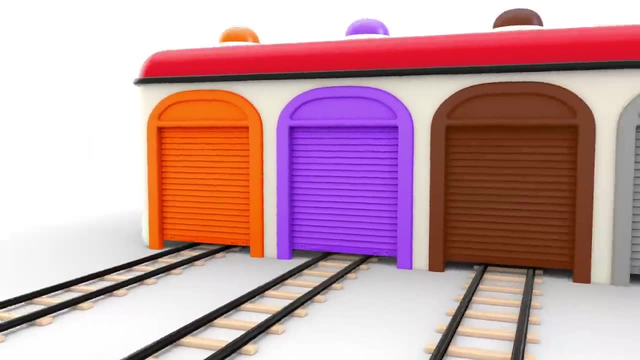 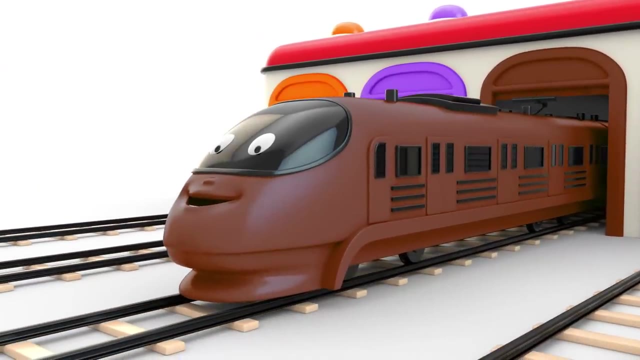 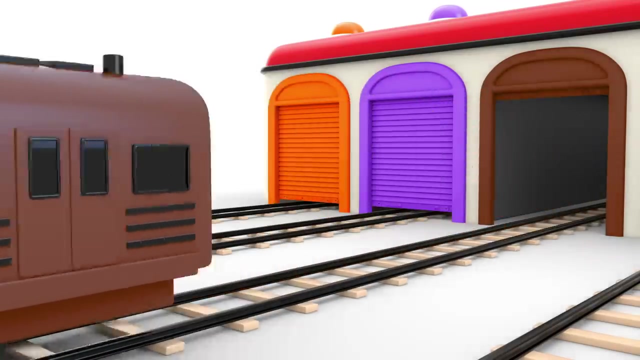 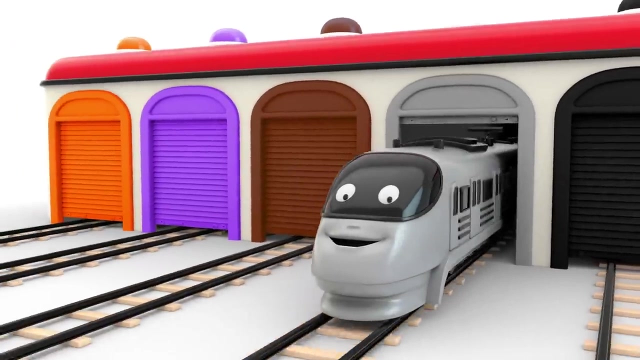 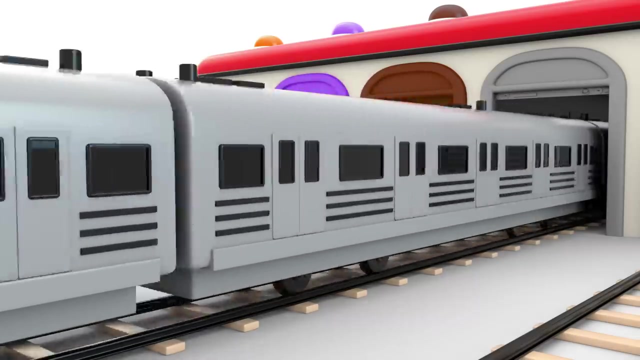 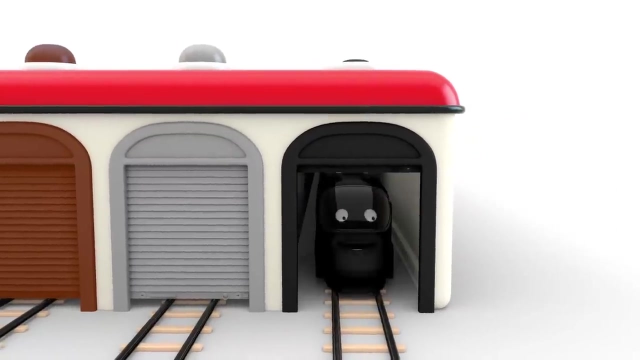